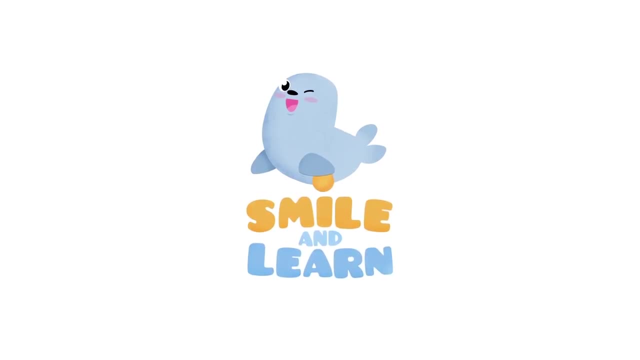 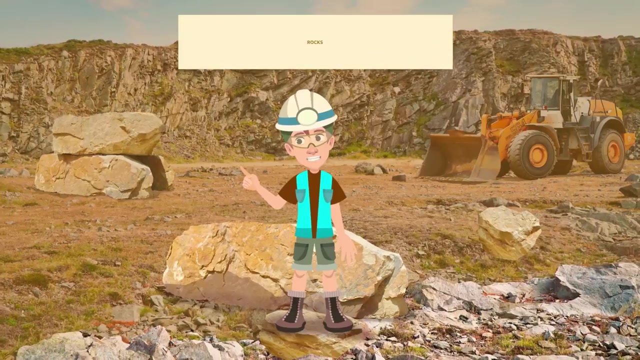 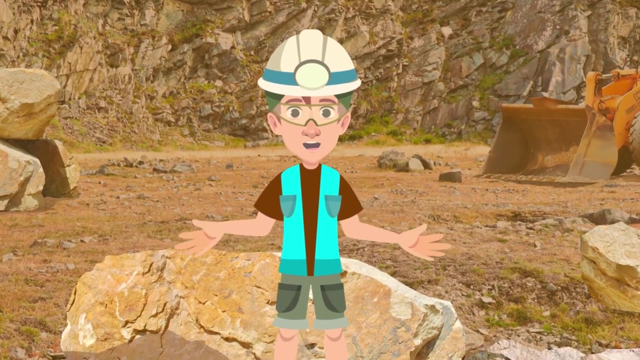 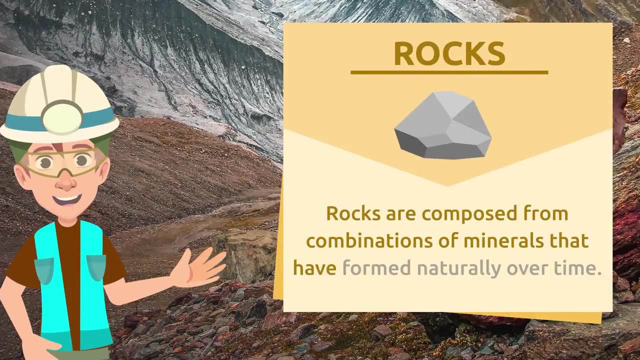 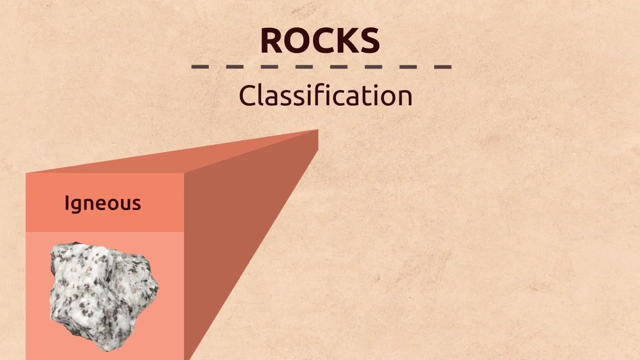 Hello friends, Today we're going on a field trip to learn everything about rocks. I'm sure you've seen thousands of them, but do you know how rocks are formed and what are their characteristics? Let's find out more about them. Rocks are composed from combinations of minerals that have formed naturally over time. On the basis of their origin, rocks can be classified as igneous, sedimentary and metamorphic. 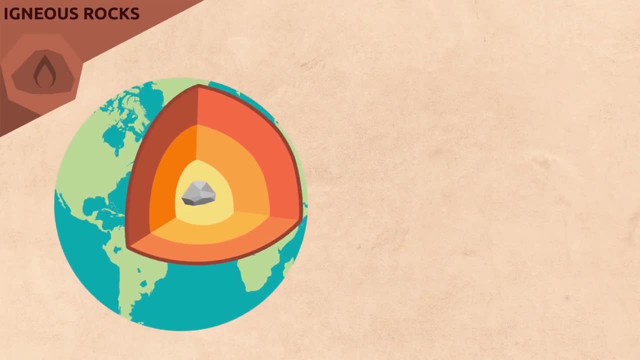 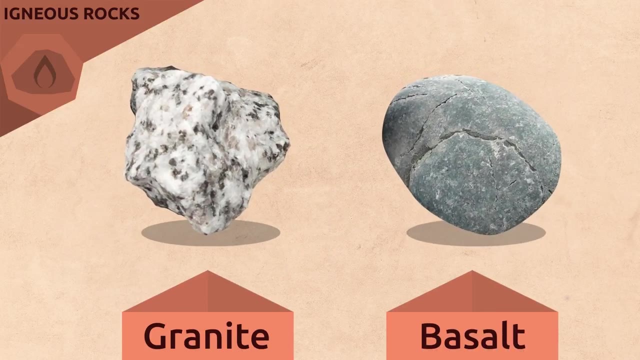 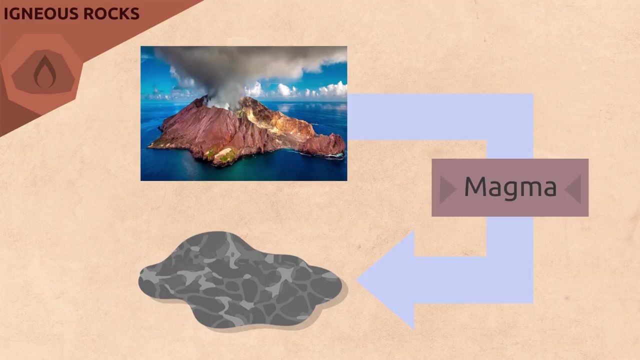 Igneous rocks are very hard rocks formed deep inside the earth. Examples of igneous rocks are granite or basalt Basalt. Both are formed from magma which erupts as volcanic lava. As soon as it reaches the surface of the earth, lava cools and solidifies rapidly. 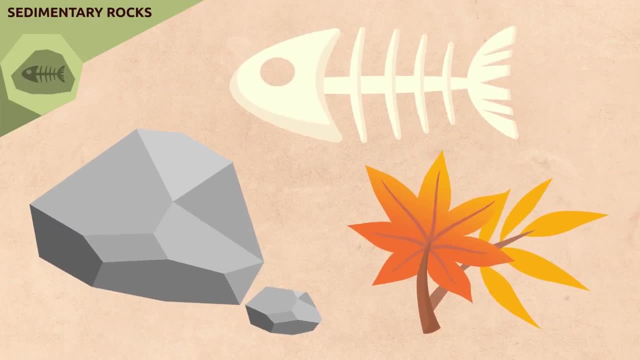 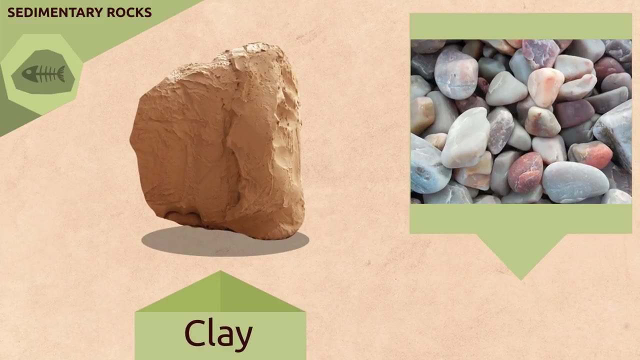 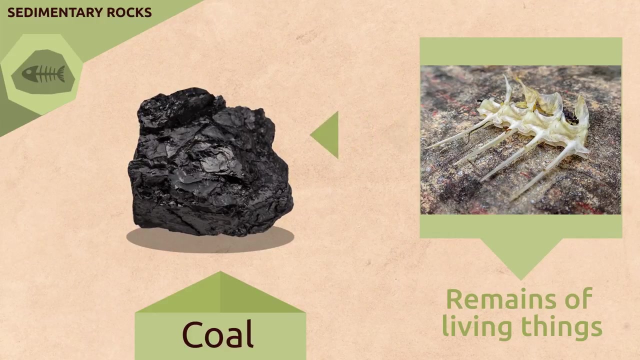 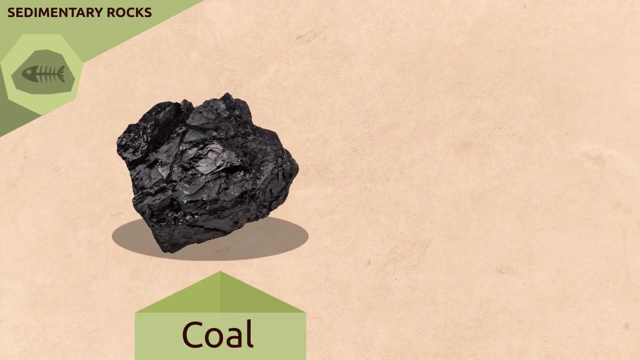 Sedimentary rocks are formed from pieces of other rocks or even once-living organisms. Clay, for example, is formed by broken up pieces of other rocks. Coal and petroleum are formed from the remains of living things like animals and plants, and from sediment deposits found in marine beds. 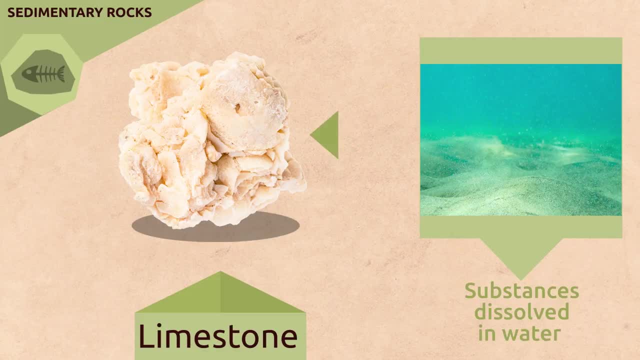 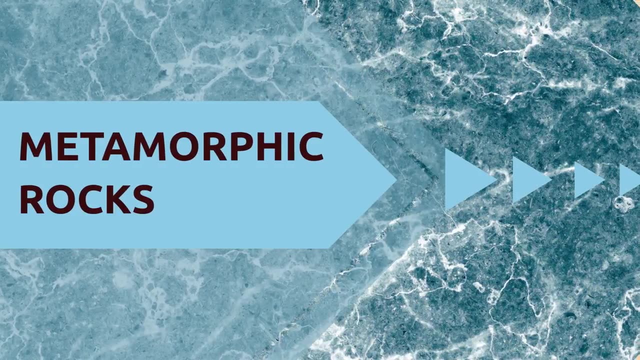 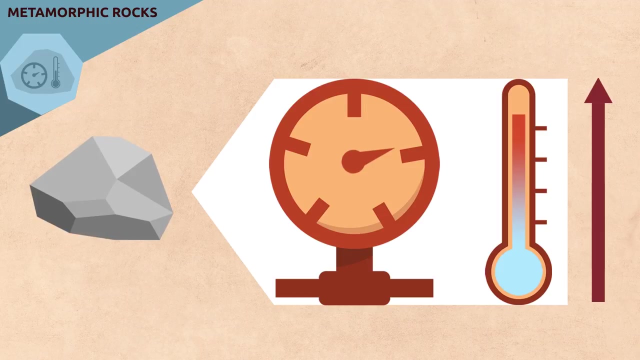 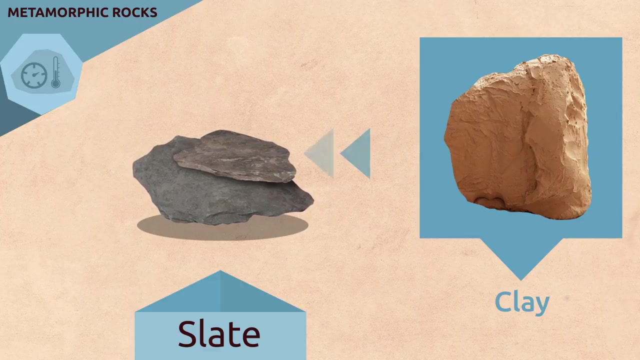 Limestone is formed from substances dissolved in water. And, lastly, metamorphic rocks that are formed by the transformation of other rocks under great pressure or heat, Like slate, for example, which is formed from clay, or marble formed from limestone. 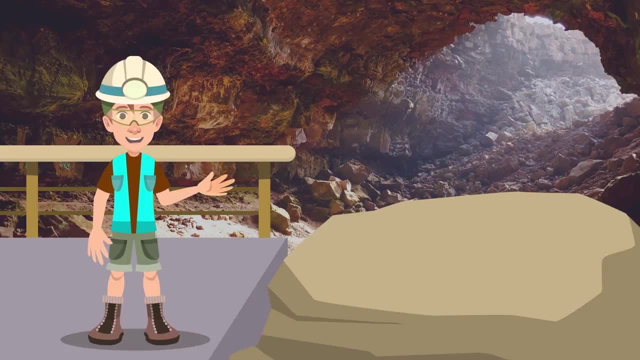 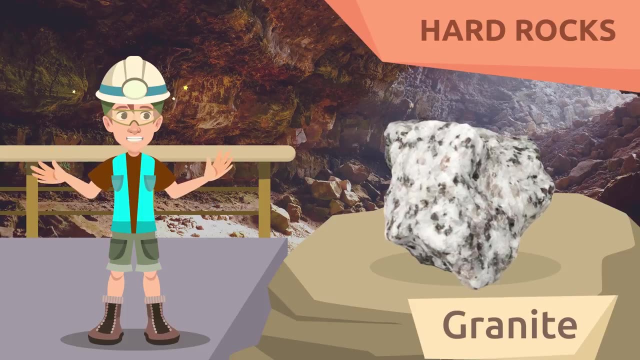 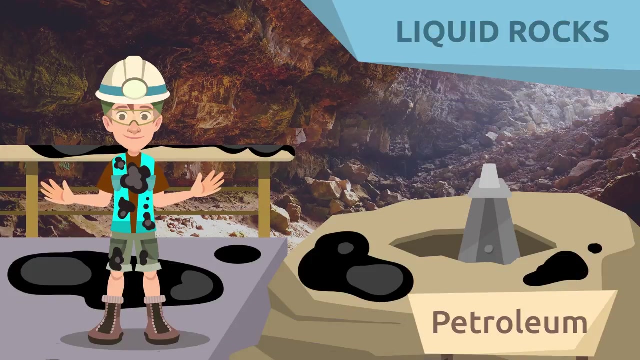 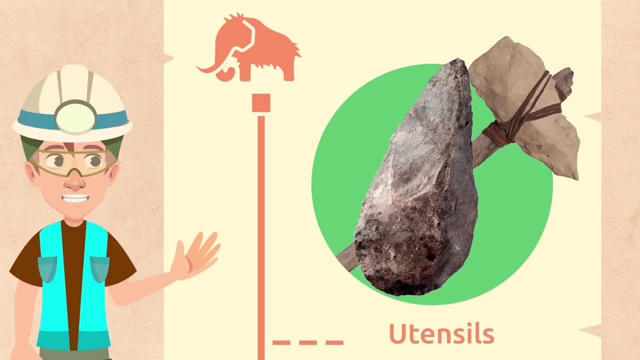 Rocks can also be classified based on their hardness. That's why we say that there are hard rocks like granite, soft rocks like clay. Petroleum is also considered a rock. Since prehistoric times, people have used rocks for a number of things like making utensils. 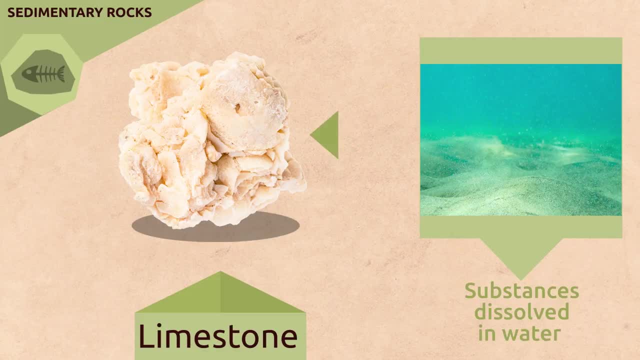 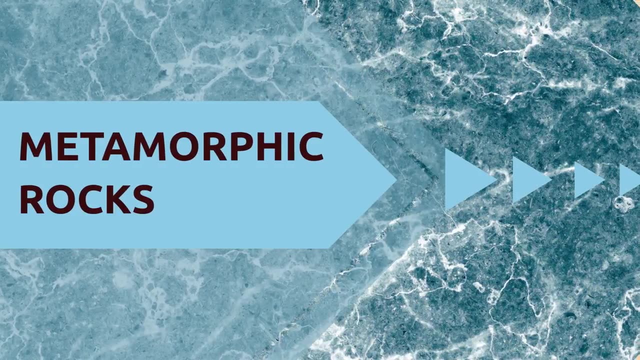 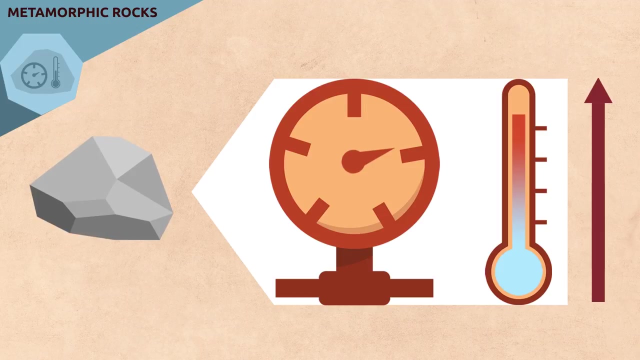 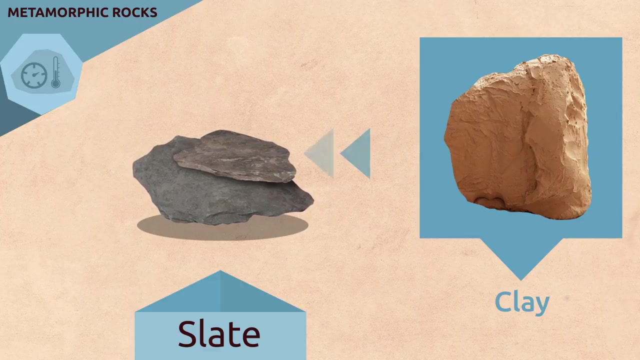 Limestone is formed from substances dissolved in water. And, lastly, metamorphic rocks that are formed by the transformation of other rocks under great pressure or heat, Like slate, for example, which is formed from clay, or marble formed from limestone. 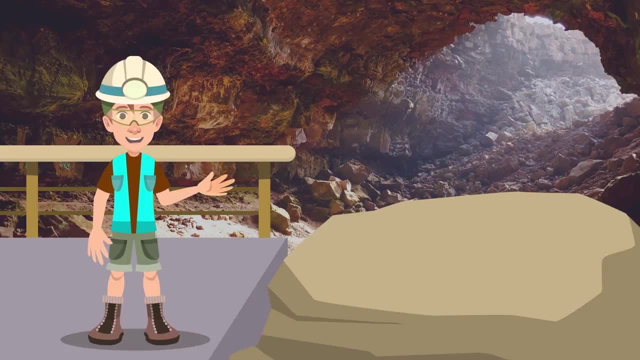 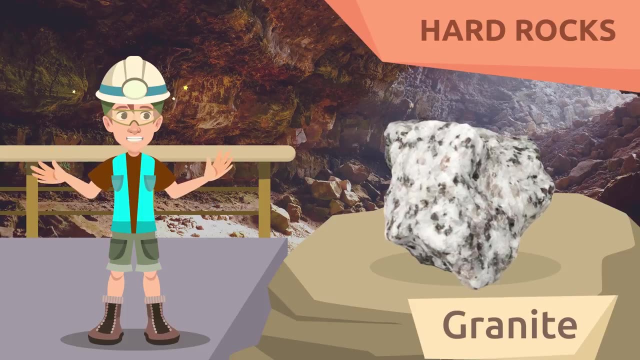 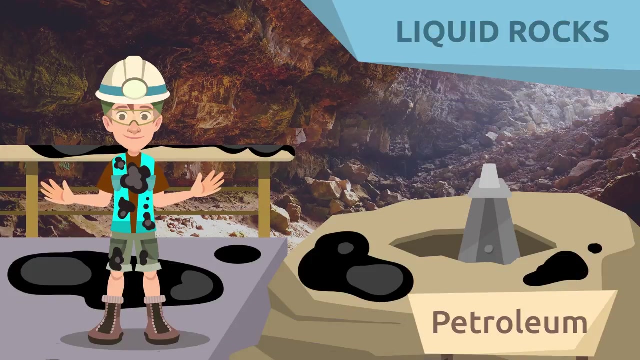 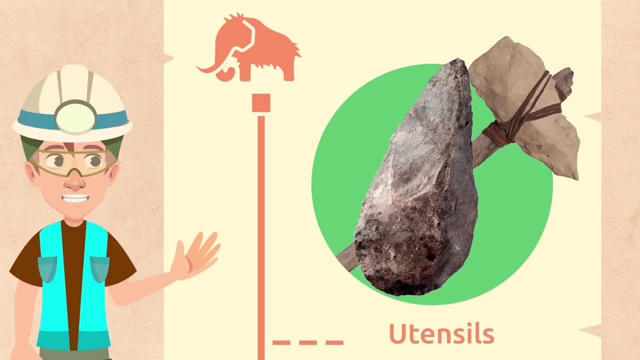 Rocks can also be classified based on their hardness. That's why we say that there are hard rocks like granite, soft rocks like clay. Petroleum is also considered a rock. Since prehistoric times, people have used rocks for a number of things like making utensils. 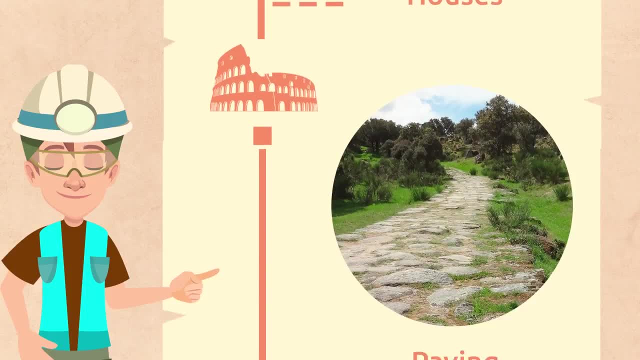 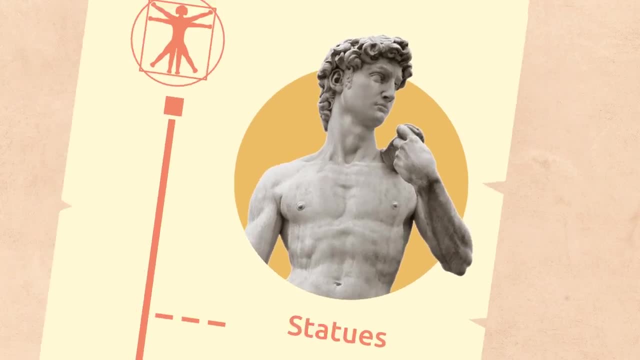 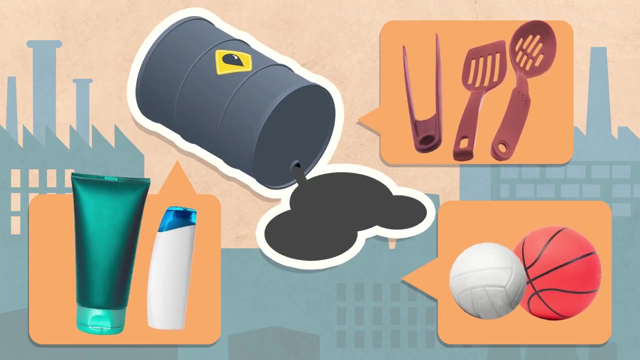 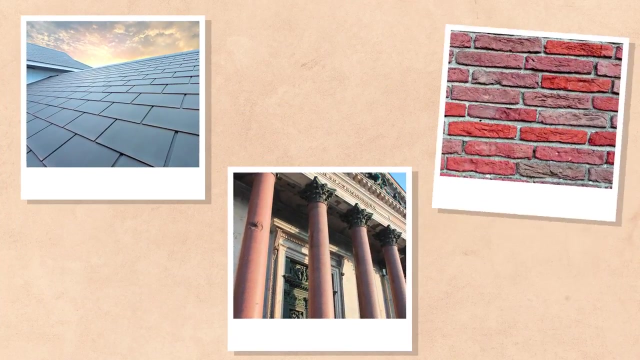 building their houses, paving or even sculpting beautiful statues like this one. Nowadays we use petroleum in different industries for making plastics or coal to generate electric power. Still to this day, rocks like slate, granite or clay are used in construction. 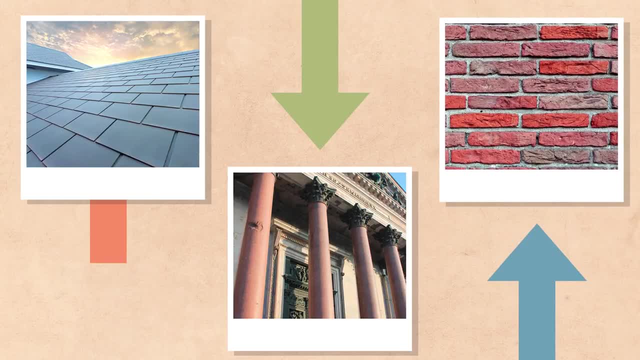 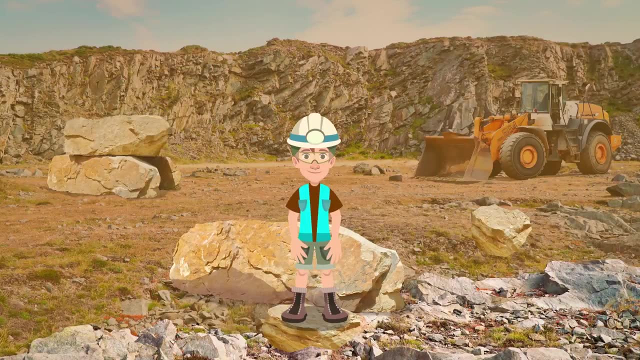 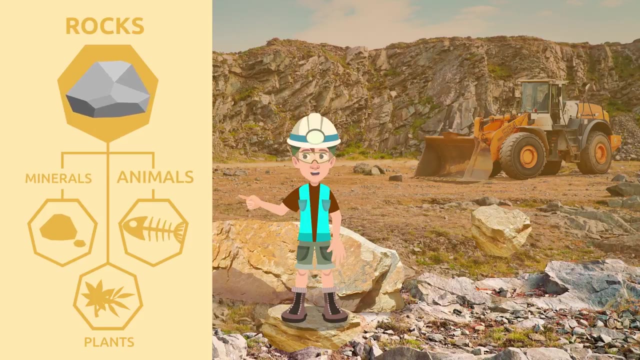 This slate roof, for example, this granite column or a clay brick. What an adventure. Today, we learned that rocks are formed from minerals or even animal and plant remains, And that, based on their origin, they're also formed from minerals and even animal and plant remains. 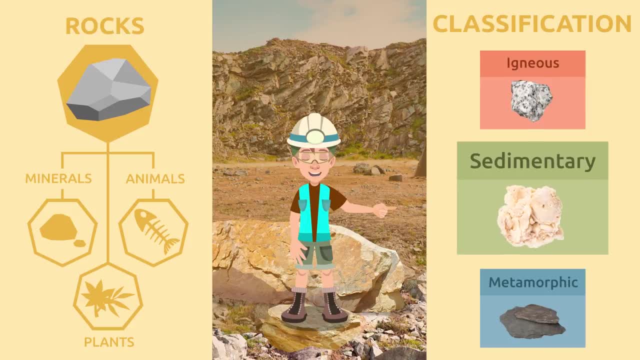 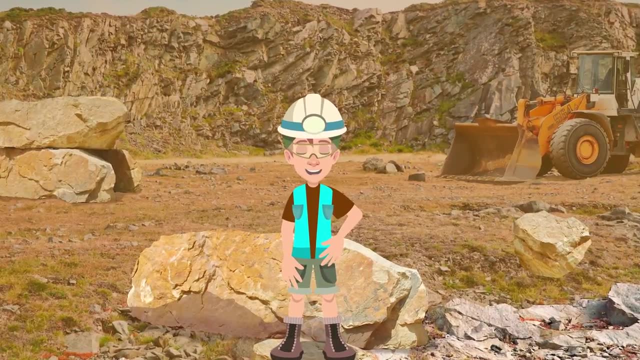 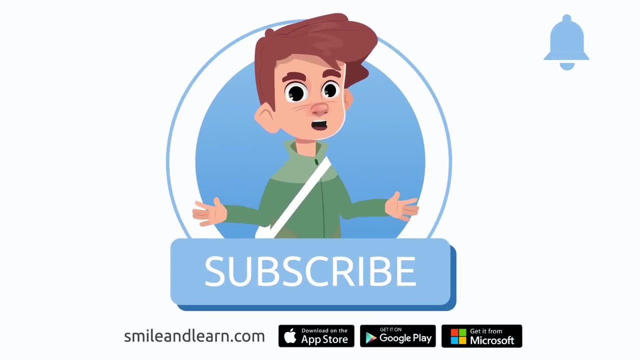 And that, based on their origin, they're also formed from minerals and even animal and plant remains. we classify them as igneous, sedimentary and metamorphic Rocks are everywhere and play a major role in the world around us. At the same time.